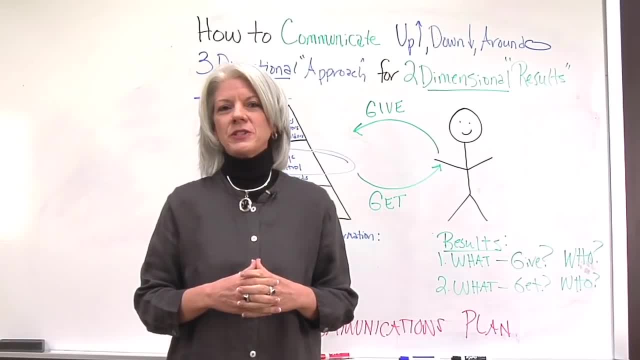 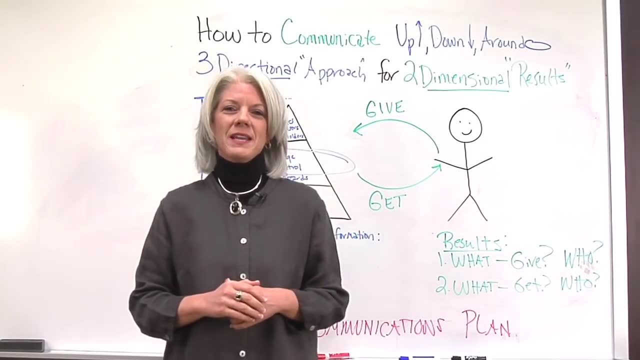 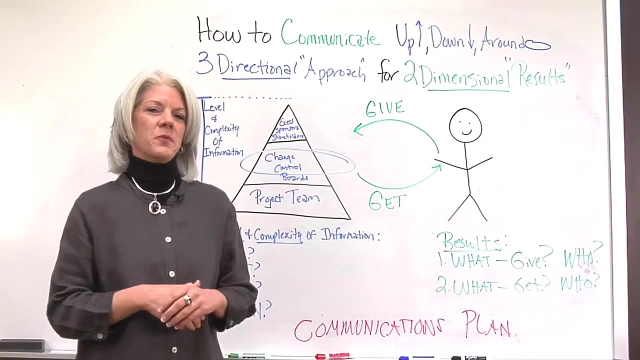 we get calls When we go in to talk with organizations, it's the most talked about. it's the most communicated issue that there is on projects. It's communication. So we can look at it at multiple angles. Today, what we want to look at on this whiteboard session is looking at all angles, One common: 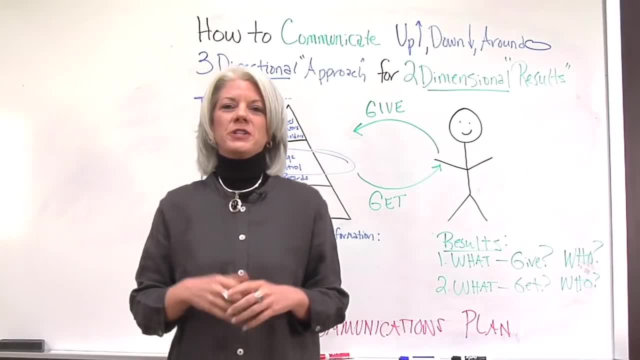 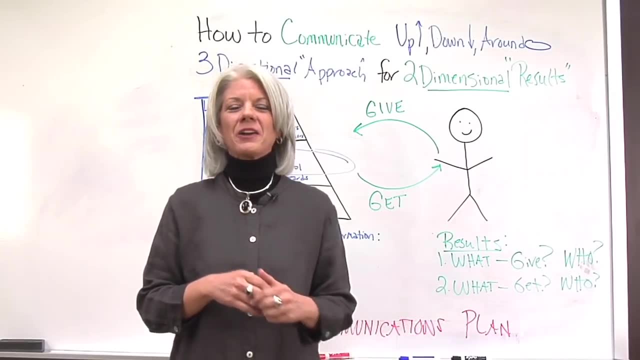 complaint we get from executives is they get too much information and they can't really cull through the information to find out what is the true status of the project. Are we on track? are we off track? are we on the right track? Are we on budget? are we off budget Then? likewise, at the same time, we have complaints. 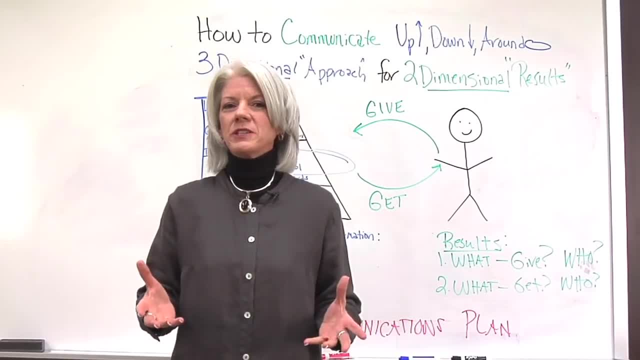 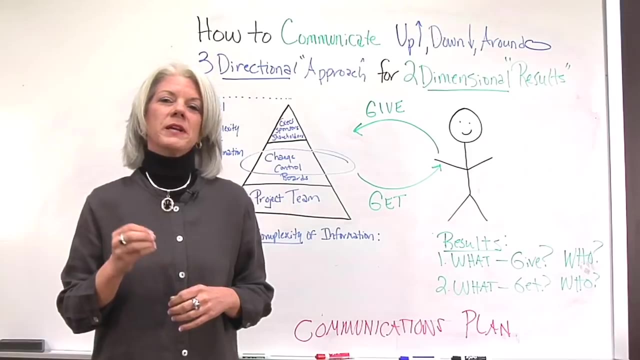 about the project level not getting enough information so they know what's been completed, what dependencies are impacting their deliverables. So a lot of times it can be a big ugly mess And we're going to talk about the components of some of the communications plan today. 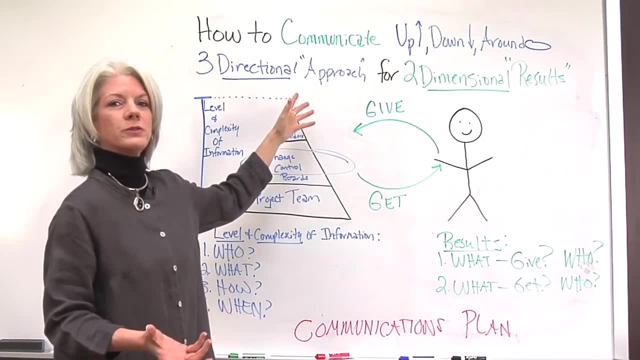 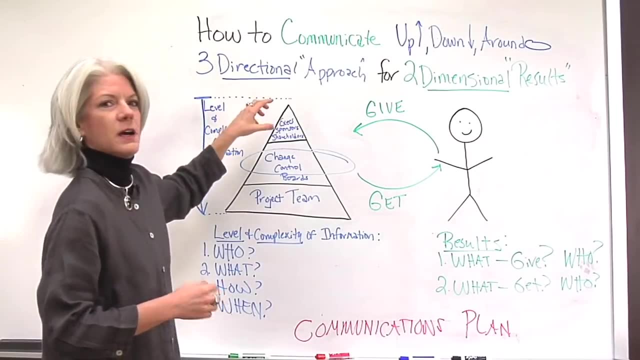 And we're going to talk about a three-directional approach For two-dimensional results. So what does that mean really? So if we look at a pyramid, the executives, sponsors and shareholders being at the top, at the peak, there are fewer. 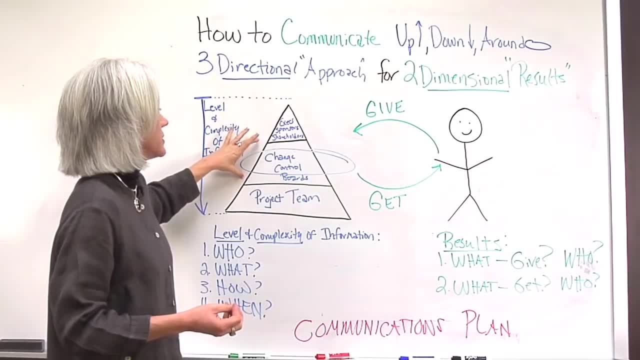 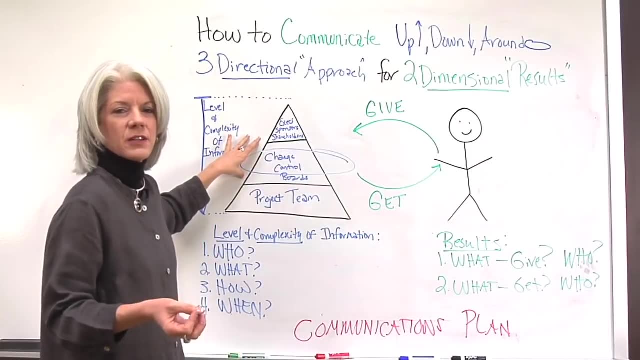 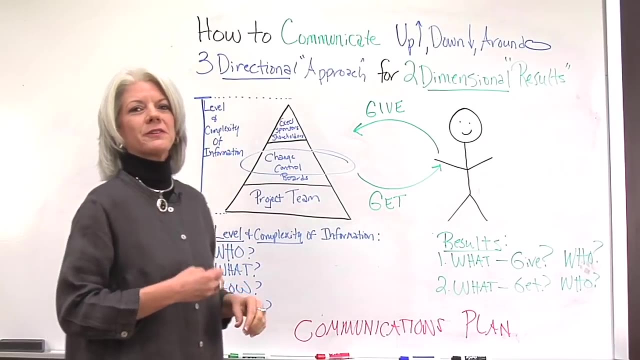 of these people on our projects. Then we go to the change control board, where there are probably more members representing maybe business units, different organizations, outside organizations, internal organizations and then project teams. Again, project teams can be internal, they can be external, They can be multiple members at multiple levels. So, as we look, 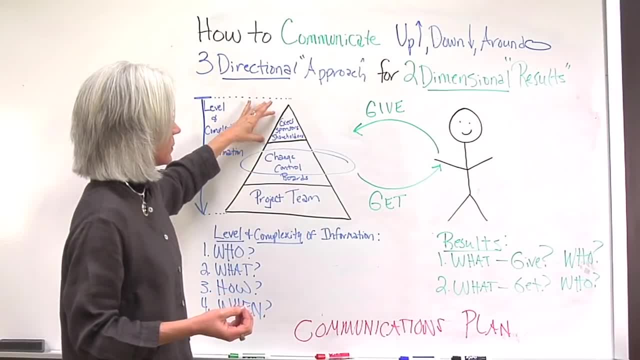 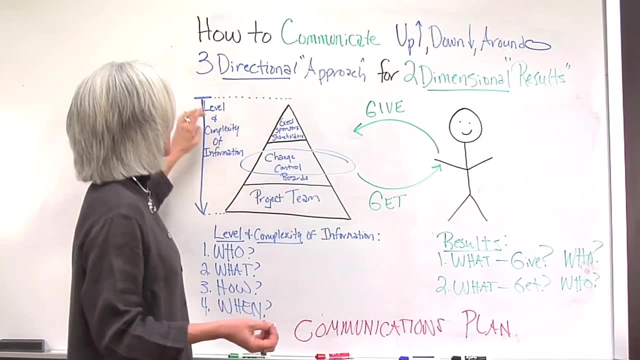 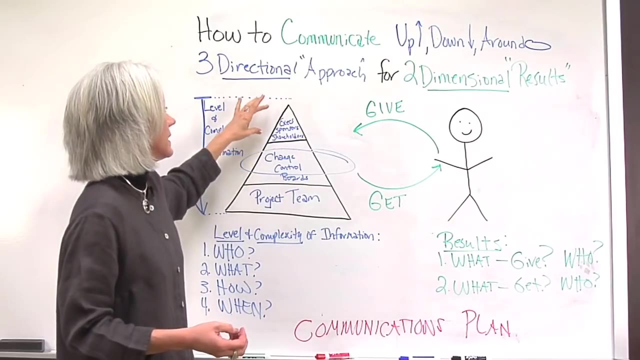 at this pyramid as the number of people- these numbers being fewer people to an increased number of people and doing different jobs- we want to look at the level of complexity of information that's required or needed is different And these people are going to need. 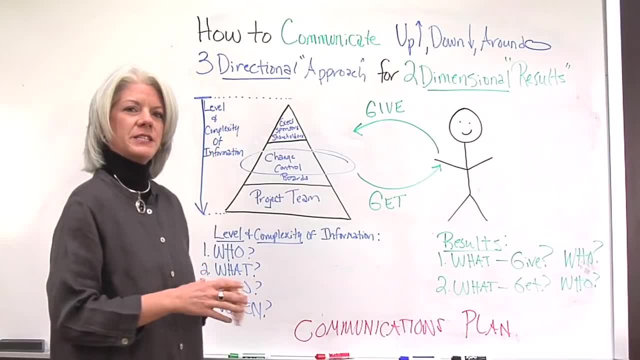 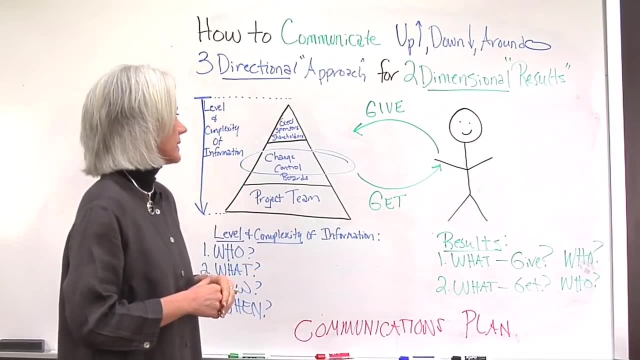 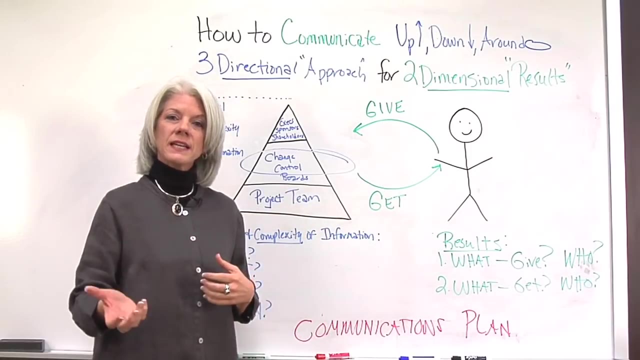 less information and less complexity. They just know that, need to know the big picture. where are we and are we on track? the change control board needs in more information to come in so that they can make decisions. make decisions, address issues, escalate issues, resolve any risk or 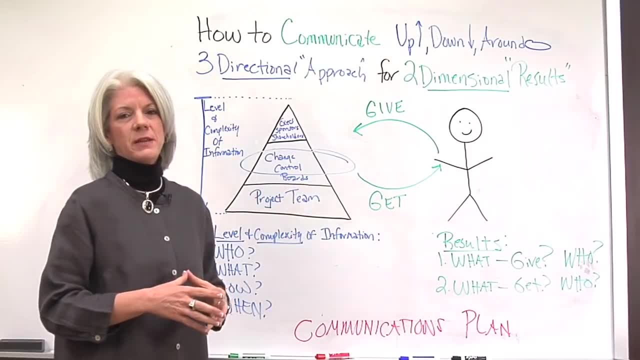 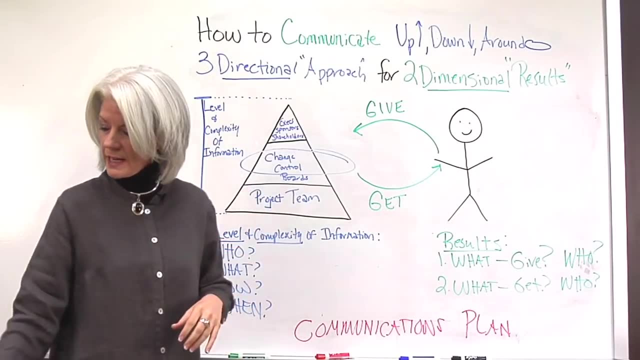 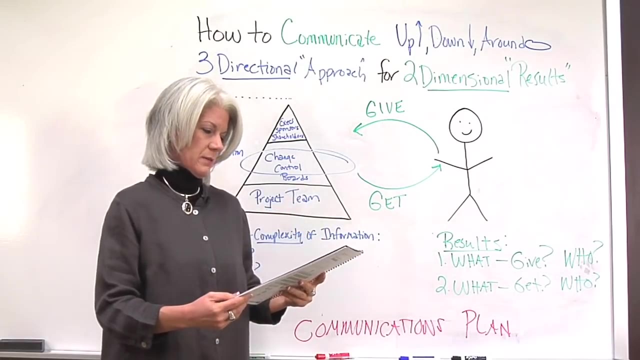 handle any change request and then the project team needing more information again so that they can complete their deliverables. so in the communications plan I brought one. so here's the literal communications plan template. I hope you have one. if not, it's always good to have a template to use. but basically in the 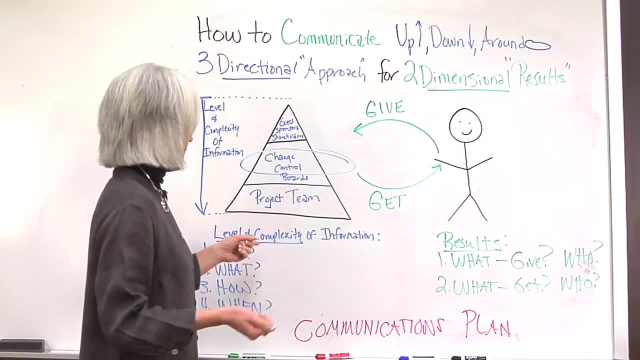 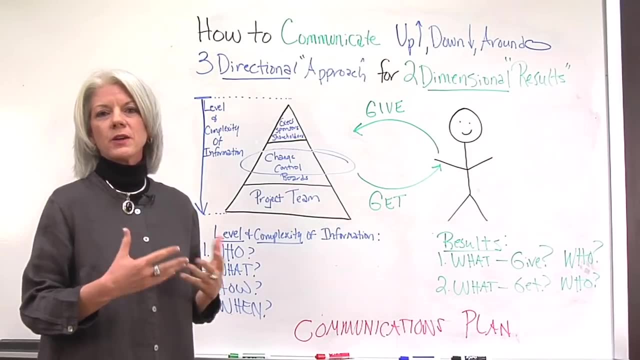 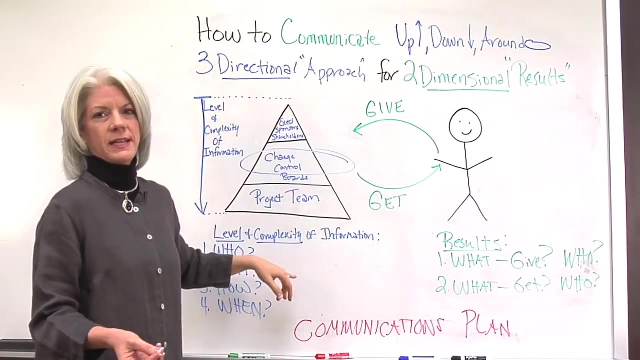 communications plan. this is the information that we have to define the level and complexity. who, who needs to know? who needs to know this information? what's their role? are they and what level? so, who is your audience? who is your audience? what information do they need that they? 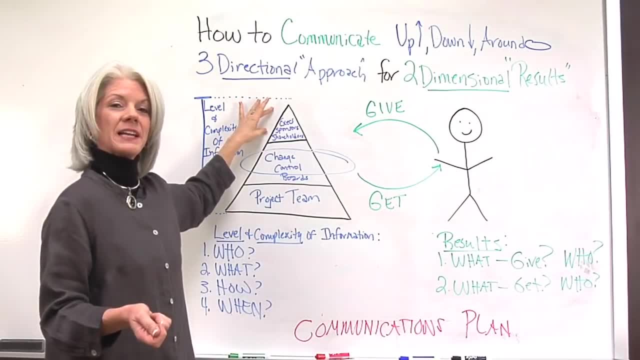 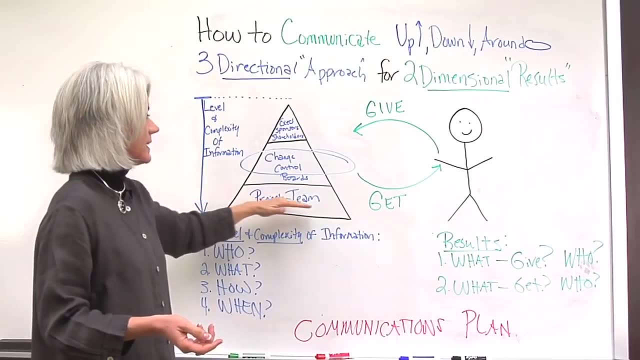 need a high level of information. and what level of information do they need? a high level status report? do they need a dashboard? do they like the red, green, yellow reports? do they like numbers? do they need budgets so that they can make decisions? do they need more information on dependencies? what do they need? how? 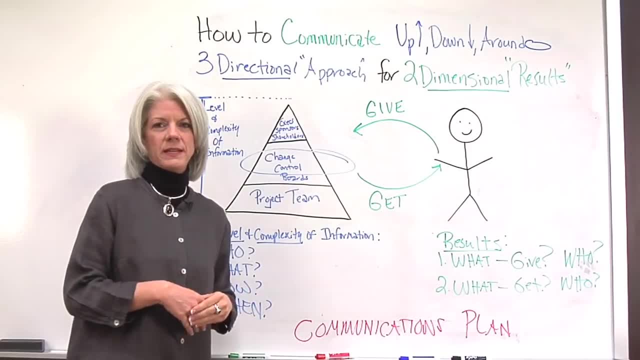 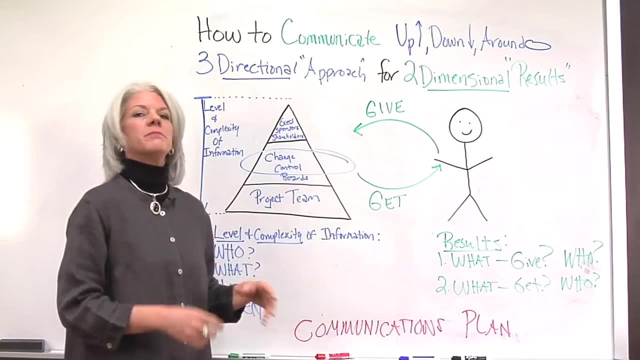 often do they need this information and how do they need to receive it? do they need to receive it in a dashboard, a weekly report, a monthly report that? do they need it by email or some online system? how are they going to get that information and how often? 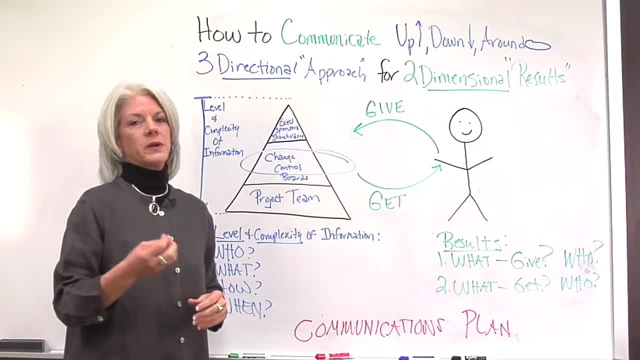 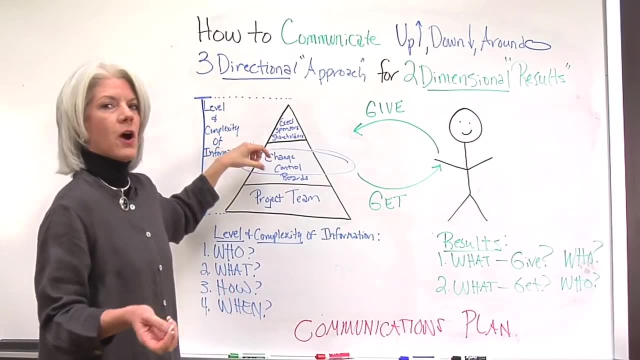 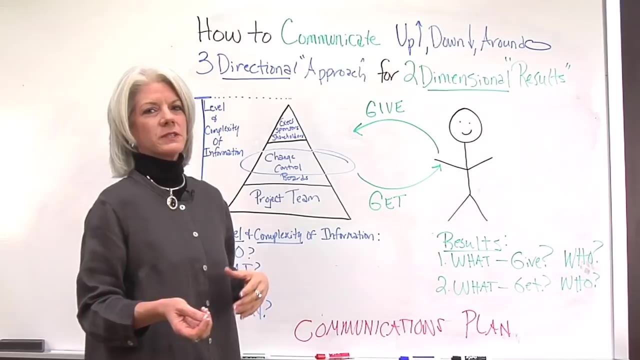 and when. again, the frequency: how frequent are they going to get this information? so then we look at, that's the directional approach, knowing your audience, and then here you are, the project manager, here you are, and to remember the results, the results being there. two-dimensional, it's a giving and 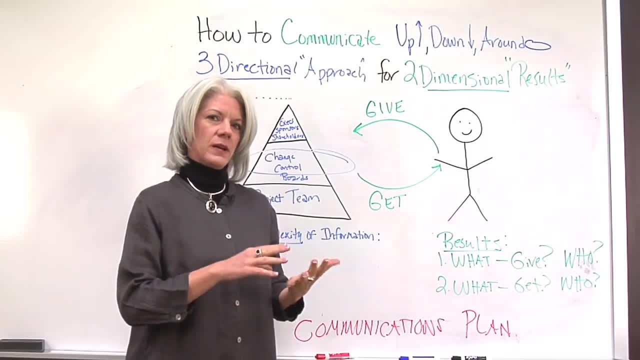 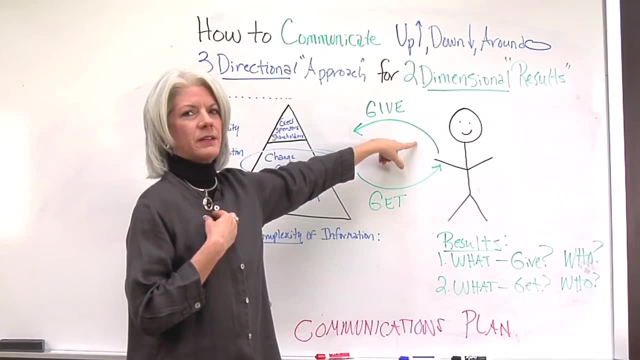 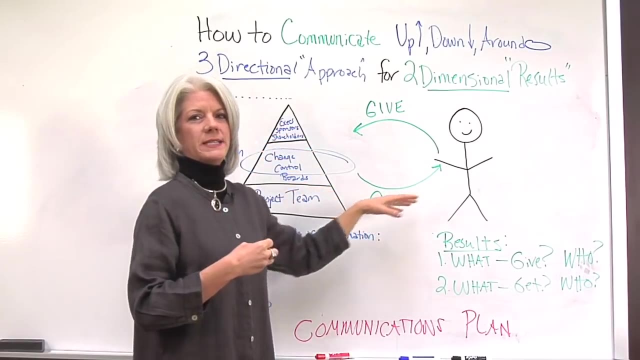 it's a getting. so going into any kind of meeting or any information you need, you, as the project manager, need to know what information do I need to give my audience, these groups of people, what information do I need to get give and what do I need to get back? a lot of times we go through and we forget. 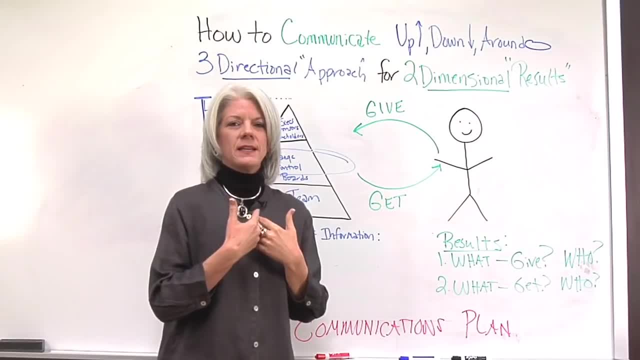 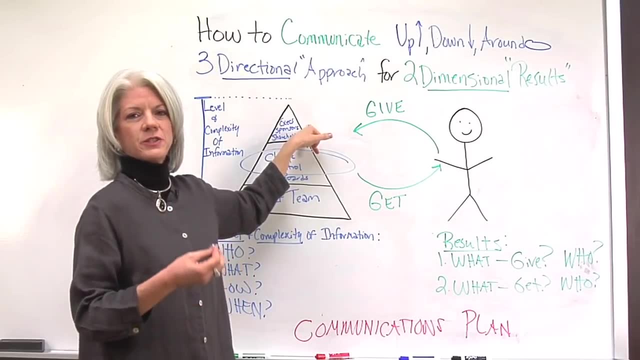 that we're just calling out information, but it's important that we get information that we need from these people. we need- may need- some decisions. they may need decisions. is this project still a priority? where are we on the priority list? what kind of business-wide decisions are?